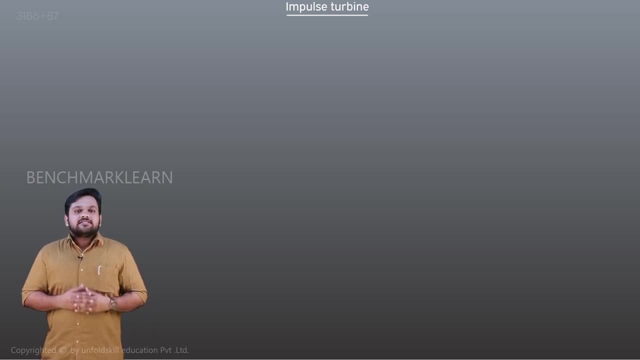 Impulse turbine. To understand the working of an impulse turbine, first let us understand what is impulse. Impulse is defined as the force acting on a body for an instantaneous period of time. It is also defined as change in momentum. Now let us see how this principle is applied in an impulse turbine. 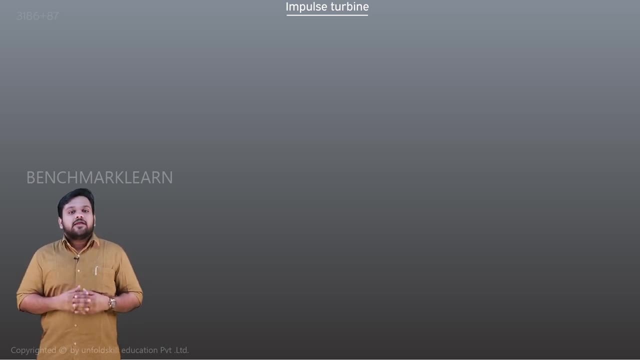 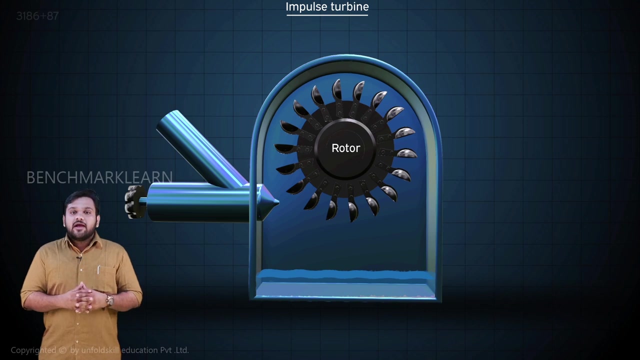 The best and foremost example of an impulse turbine would be the Pelton wheel. The Pelton wheel consists of a rotor with bucket shaped blades attached along its periphery. The blades are fixed in such a way that the distance between each one is of particular proportions. 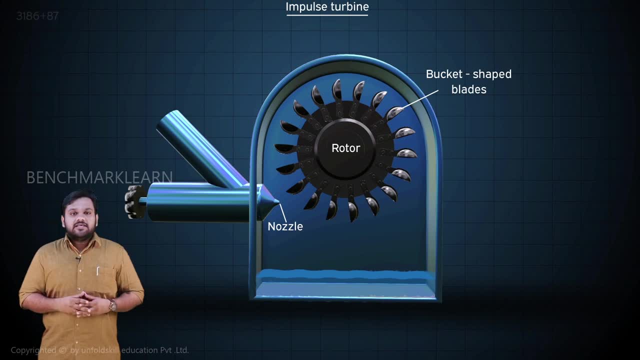 A nozzle creates a jet of high velocity. It is used to point the flow of water towards the blade. The nozzle is attached to a penstock, a pipe which extends all the way up to the water reservoir, which is usually located several meters high. 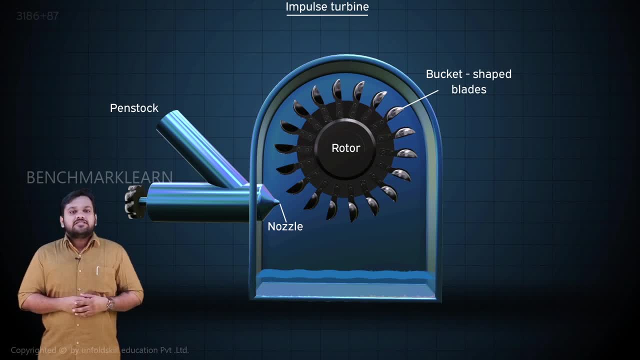 This water has a potential energy due to its high location with respect to the nozzle. This is converted to kinetic energy and hence a high velocity water jet comes out of the nozzle. Inside the nozzle there is a sphere-like arrangement which can be loosened and tightened to control the flow rate of water. 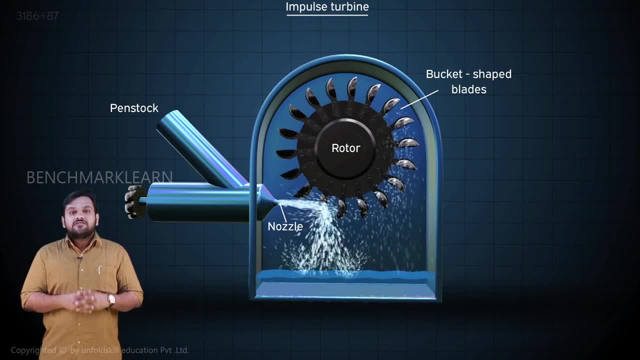 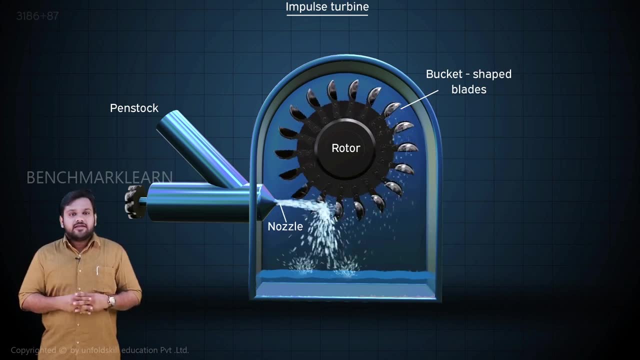 This water, when strikes the curved surface of the bucket, imparts its energy to the bucket, which in turn results in the rotation of the bucket. Due to the curvature of the bucket, the direction of the water jet is almost reversed to get maximum force. 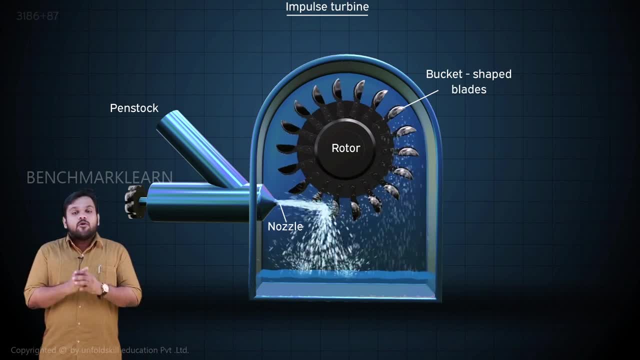 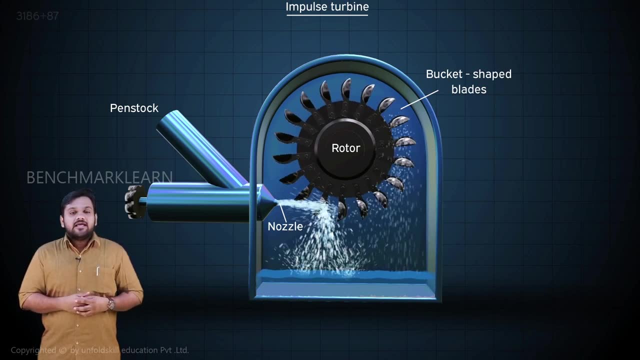 Due to the curvature of the bucket, the direction of the water jet is almost reversed. to get maximum force, The water jet's reversal is by about 165 degrees. The flow rate of water controlled at the nozzle helps in determining the speed and power generated at the rotor.